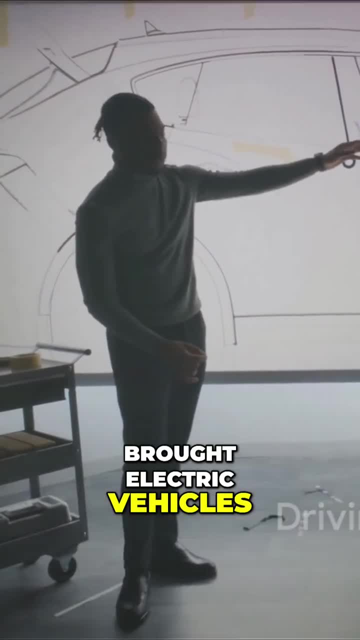 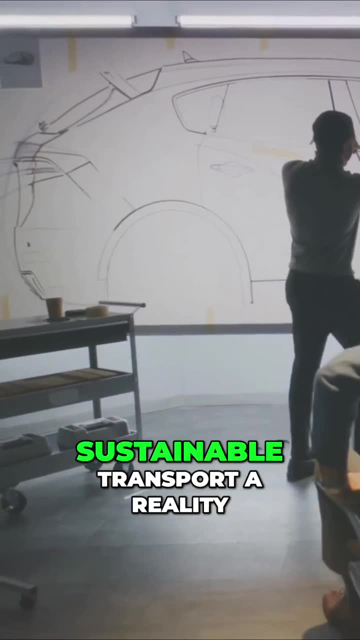 Tesla Motors, under Musk's leadership, brought electric vehicles to the mainstream market. This wasn't just about creating snazzy cars, but part of a grander vision — to make sustainable transport a reality. Tesla's innovative models, like the Roadster and Model S, broke. 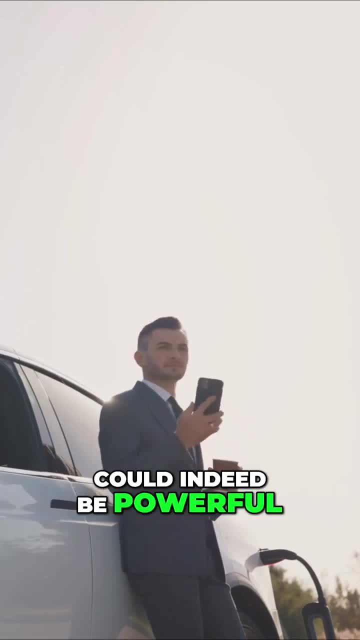 the mold proving that electric vehicles could indeed be powerful, efficient and desirable. 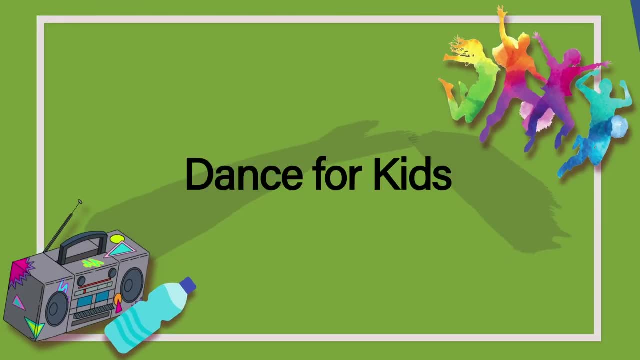 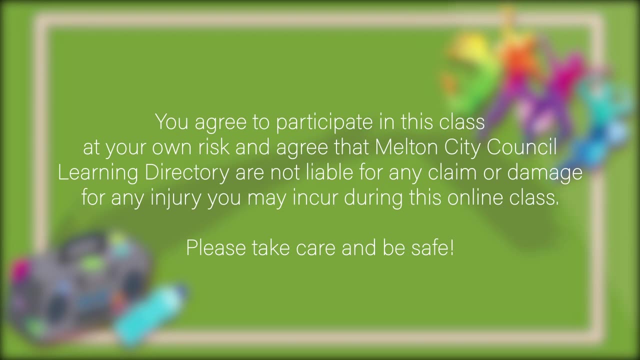 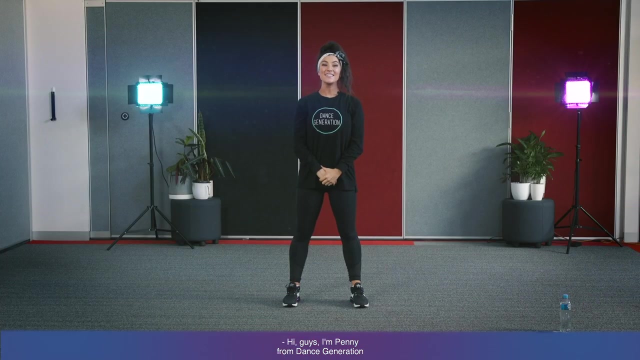 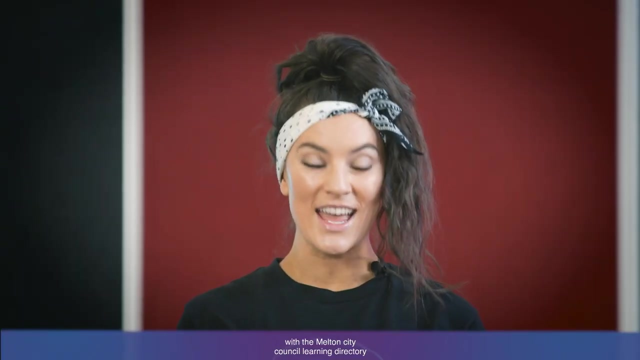 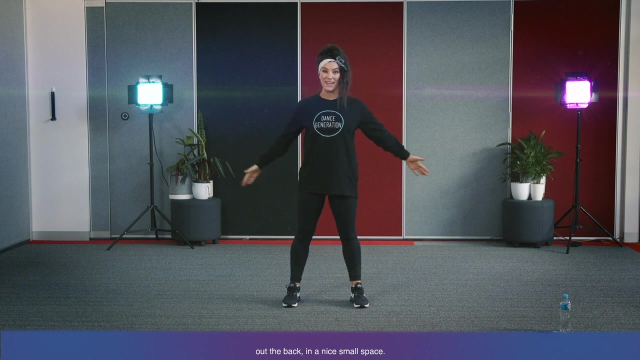 Hi guys, I'm Penny from Dance Generation Performing Arts School and today I'm here with the Melton City Council Learning Directory And today we're going to put on a hip hop class for you guys that you can do in your lounge room out the back, in a nice small space. So perhaps 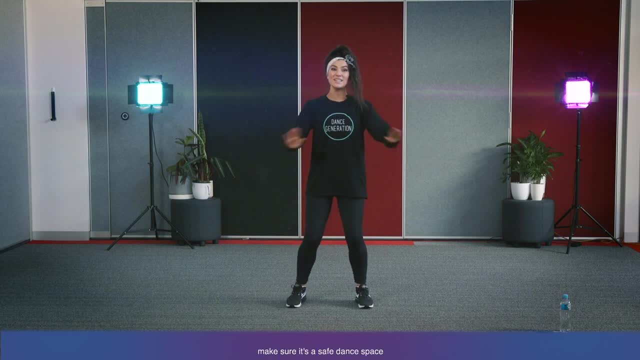 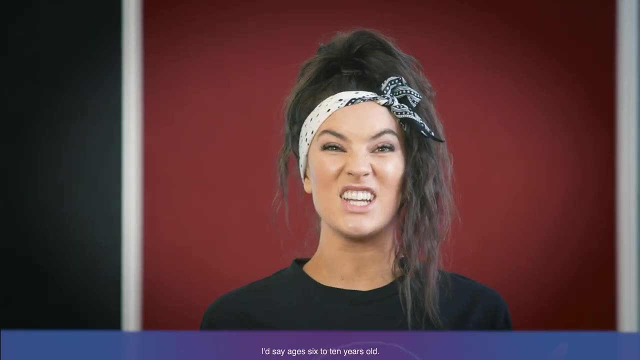 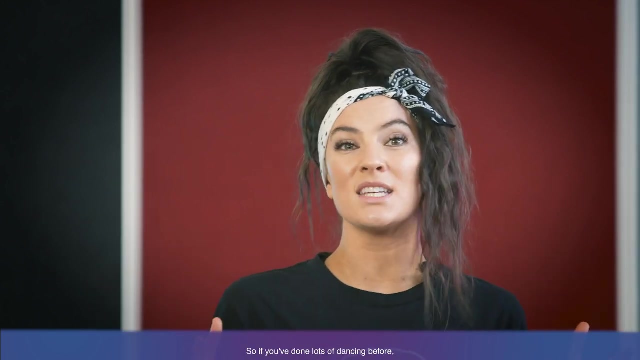 move some furniture. All we need is like a couple of metres. Make sure it's a safe dance space and you've got some room. This is going to be aimed at, I'd say, ages 6 to 10 years old. It's going to be a beginner hip hop class, So if you've done lots of dancing before, 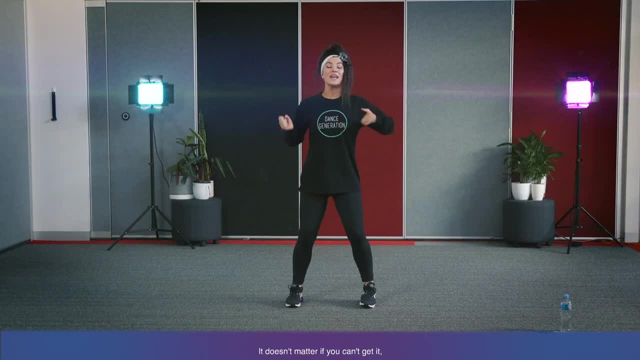 maybe it will be easy. If you haven't, maybe it will be hard, It doesn't matter. if you can't get it, It doesn't matter. I think, most of all, we've just got to get moving through this time. Let's have some. 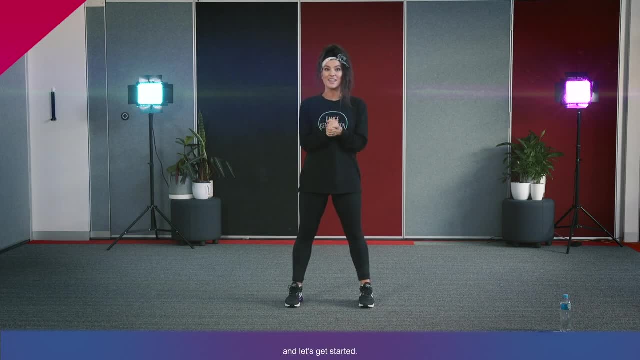 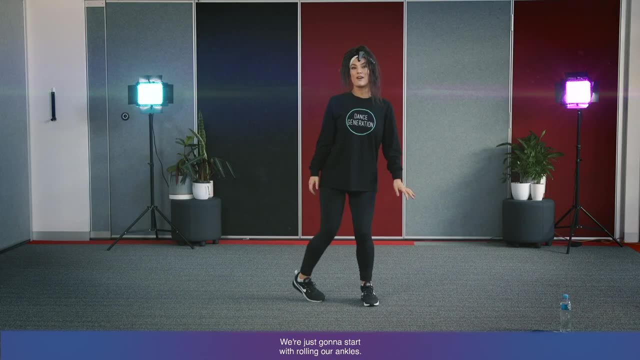 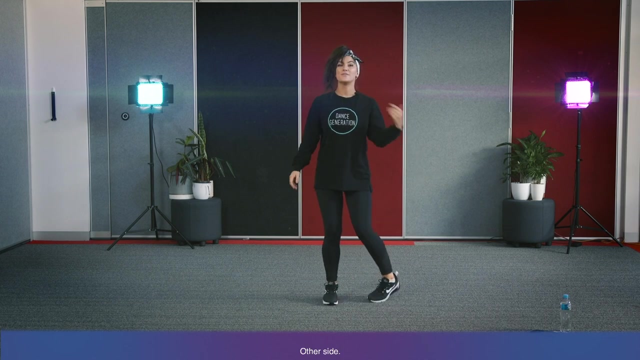